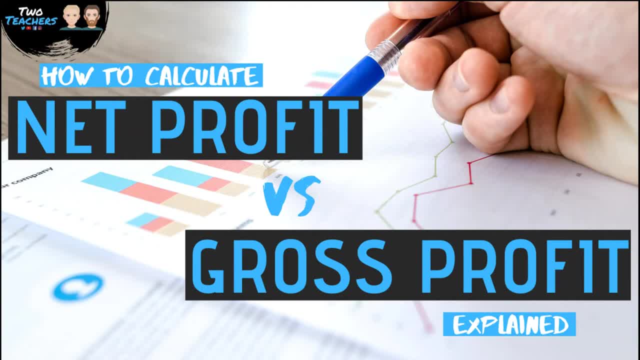 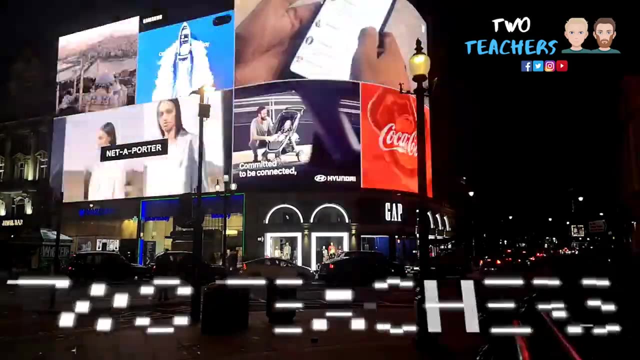 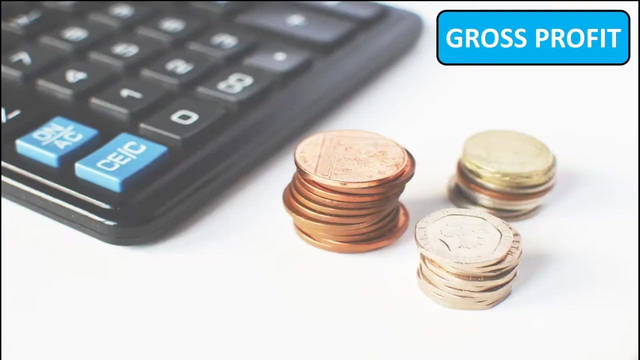 Most businesses exist to make money, and being able to calculate and interpret the net profit and gross profit margins of a business is key to measuring a business's performance. So let's take a look at how to do this. One of the most important financial concepts in business is gross profit. This is the difference. 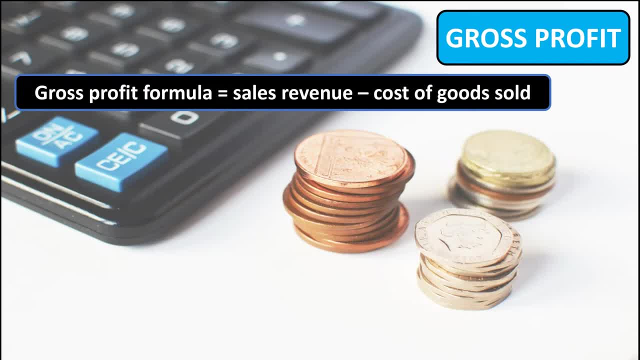 between sales revenue and the cost of goods sold. It is calculated by subtracting the cost of goods sold from sales revenue. Effectively, it's the profit a business makes after deducting the costs which are associated with making and selling its products or the costs associated. 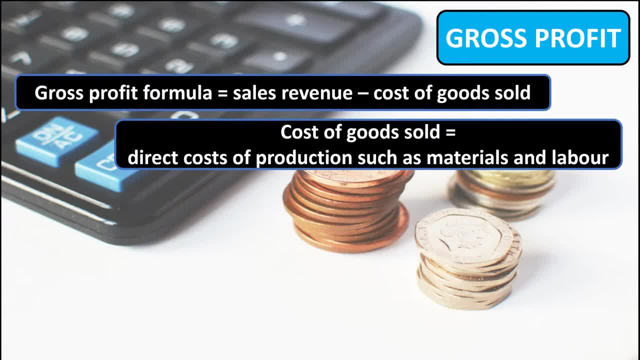 with providing its services. The cost of goods sold refers to the direct costs of producing the goods sold by the business, which includes the cost of materials and the labour which is used to create the goods. However, it's important to note that gross profit only includes 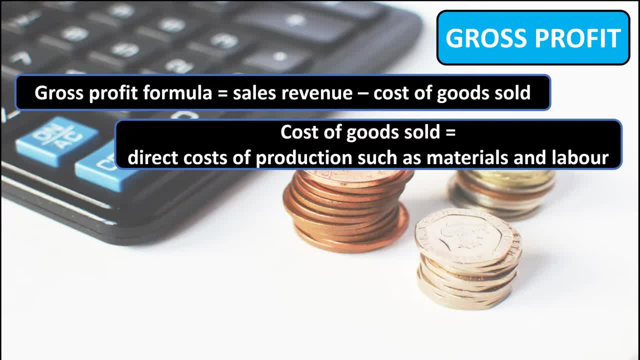 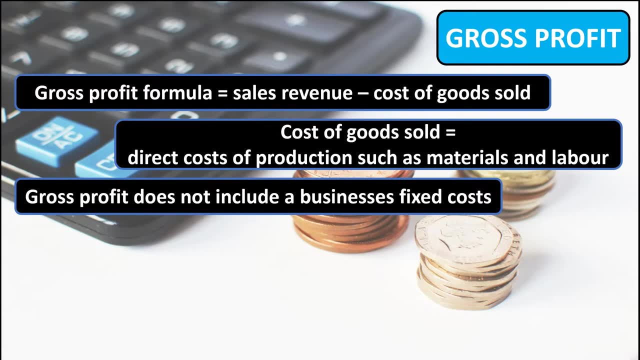 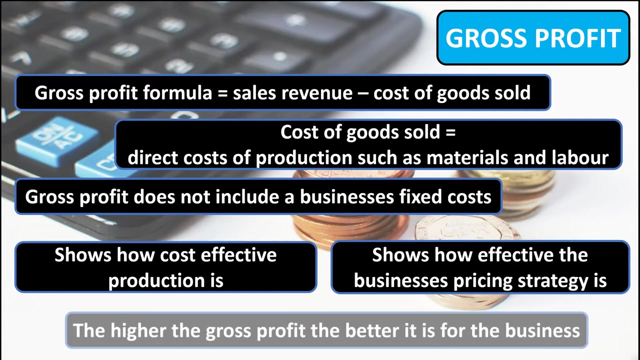 variable costs to a sales revenue. The gross profit of a business essentially shows how good they are at producing products or services at cost-effective price and how accurately they can price their products to maintain a high volume of sales with the highest possible margin. Essentially, the higher the gross profit, the better it is for the business. 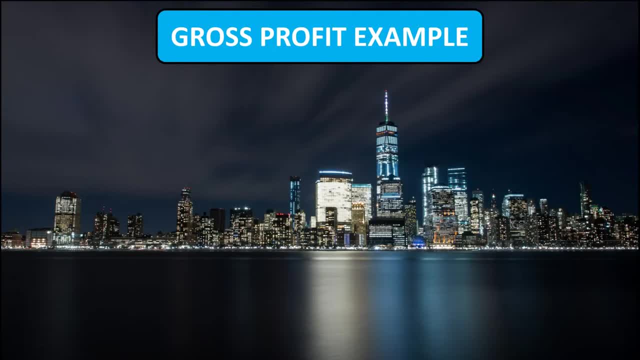 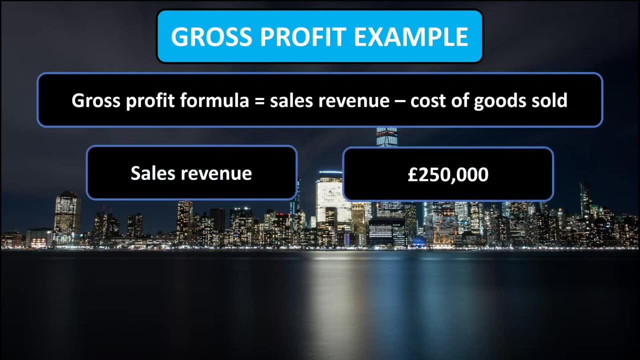 So let's take a look at calculating the gross profit Now. the figures a business requires to calculate their gross profit can all be found on their income statement. Firstly, we start with the sales revenue, which in this example is £250,000.. 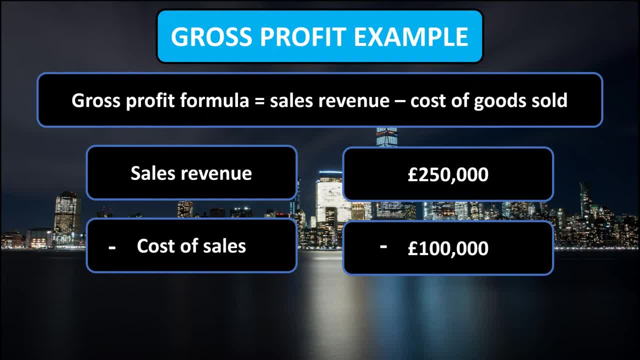 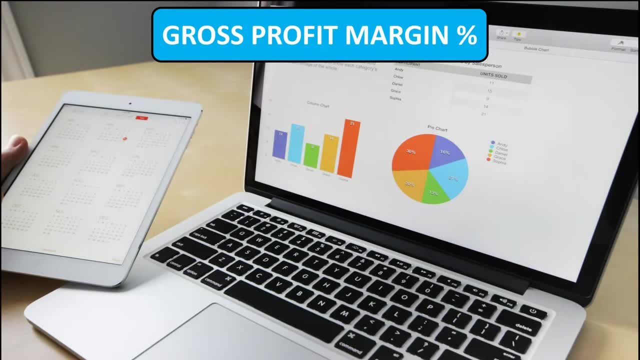 We then deduct the cost of sales, which in this example is £100,000.. This leaves us with £150,000.. This is our gross profit figure. Now, if the business has calculated its gross profit, it can now work out its gross profit. 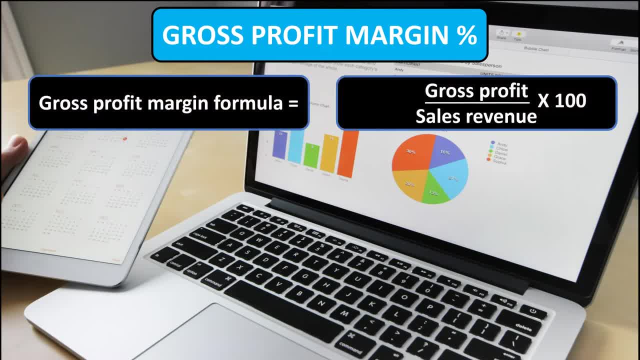 margin, which is always shown as a percentage. The gross profit margin is calculated by dividing the gross profit by the business's sales revenue and then multiplying the answer you get by 100.. So if we use the figures taken from the previous example, this would mean we would start with: 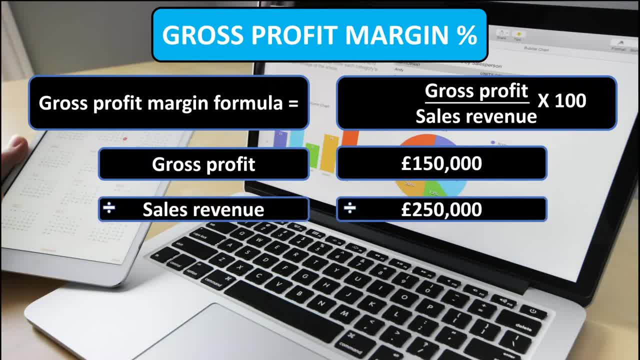 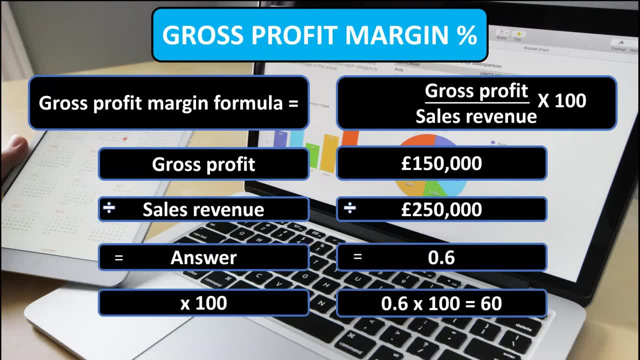 the gross profit of £150,000.. We would then divide this by the sales revenue of £250,000.. This gives us an answer of 0.6.. Now it's very important to remember to multiply this answer by 100 to turn it into. 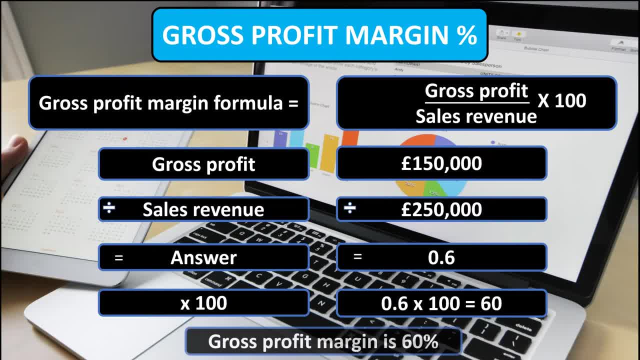 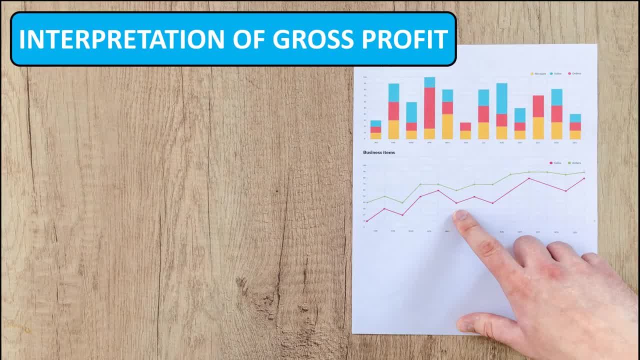 a percentage which, in this example, gives us 60. This is the gross profit margin. So 60% of this business's sales revenue is gross profit. What's classified as a good gross profit margin will vary depending on the business and the industry it operates with in, So let's have a look at how to interpret the gross profit. 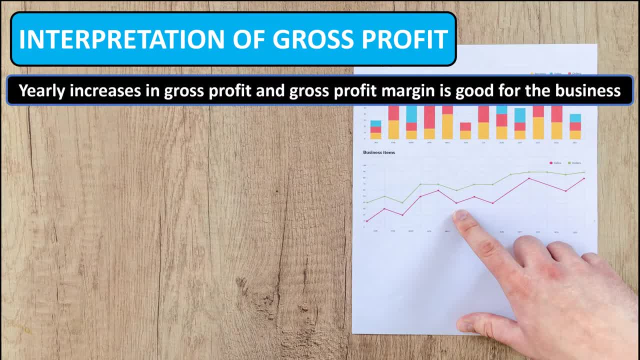 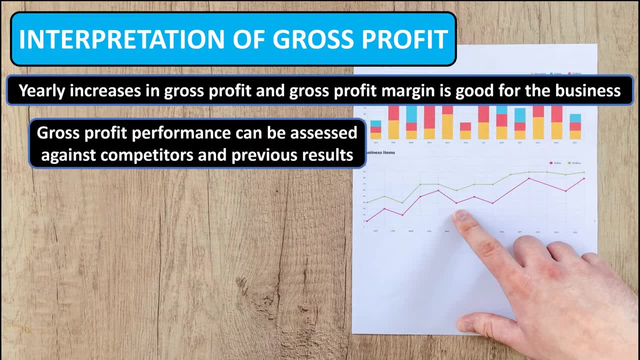 of a business. Put simply, businesses want to see their gross profit and gross profit margin increase year on year. The higher it is, the better for the business. One key way to assess gross profit is to compare it with competitors. if this information is available Another way, 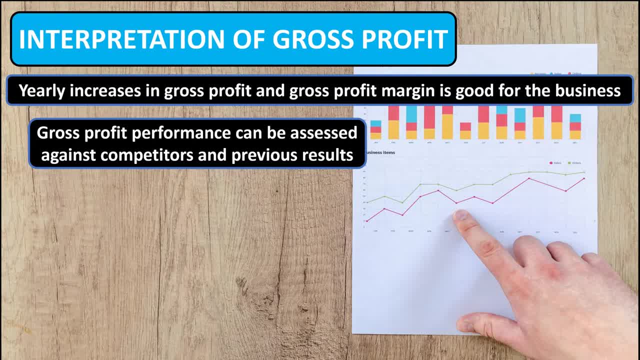 is to compare the gross profit margin against previous years to see if it is increasing or decreasing. If a business's gross profit margin is decreasing year on year, then this must be investigated by the managers and owners of the business to resolve the issue as soon as possible. 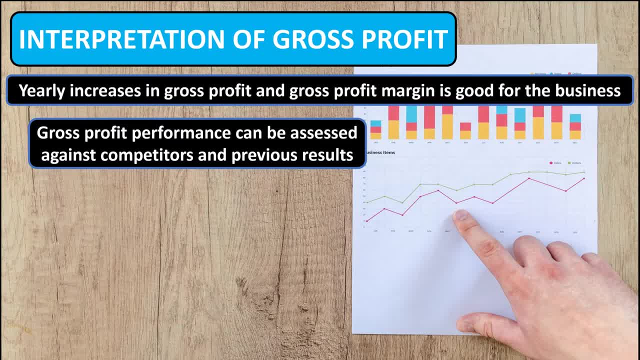 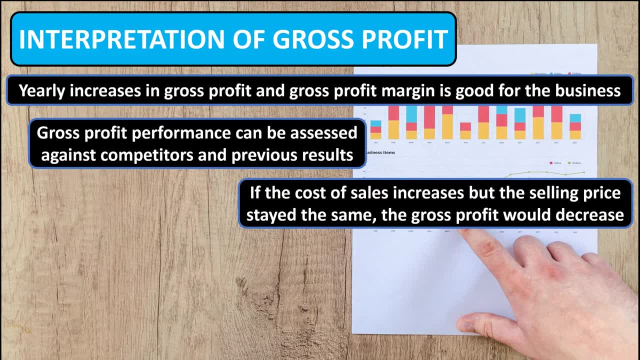 If this was the case and the owners wanted to investigate a change in the gross profit, typically consider a few key factors. to begin with, One reason for a change in the gross profit could be linked to the cost of sales. If this figure was to go up, for example, the materials for producing a product or the labour pay. 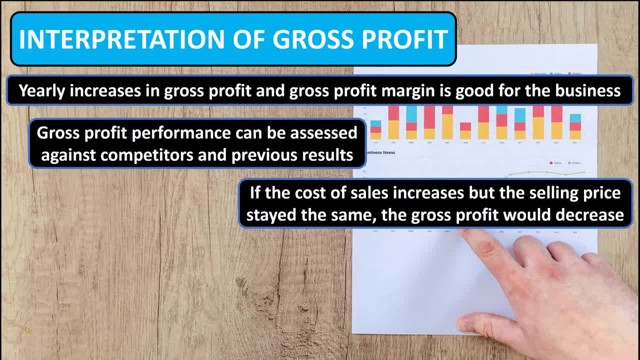 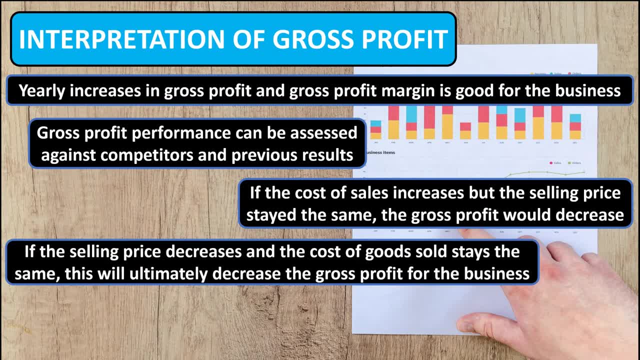 per hour increased, but the selling price stayed the same, then the gross profit of the business would decrease. A second key reason for a change in a business's gross profit is the price at which products are being sold. If the business's products are now being sold at a lower price and the 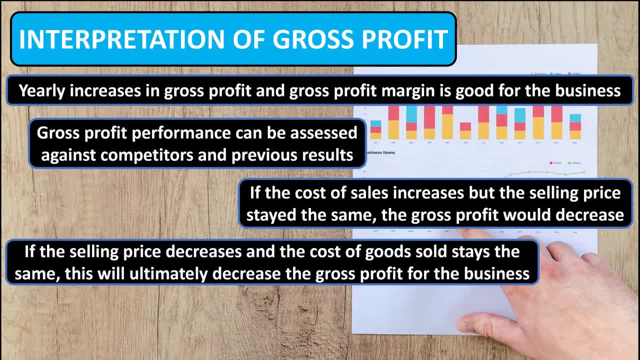 variable costs remain the same, this will ultimately decrease the gross profit margin. This is a key reason for a change in the gross profit could be linked to the cost of sales. Another reason for a change in the gross profit could be linked to the price at which 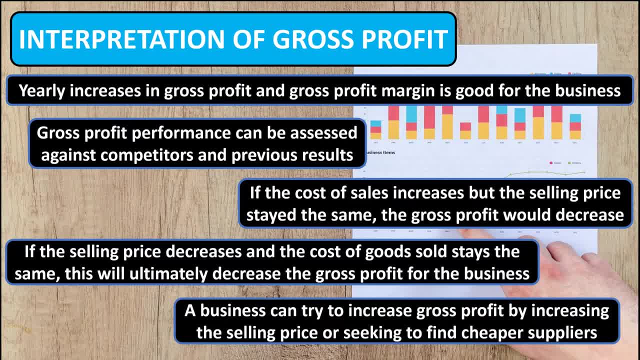 products are being sold. Once a business has investigated and found the reasons for the change in gross profit, it can implement change, For example, increasing the selling price or seeking to find cheaper suppliers. So now we're going to move on to net profit. This is sometimes referred to as the bottom. 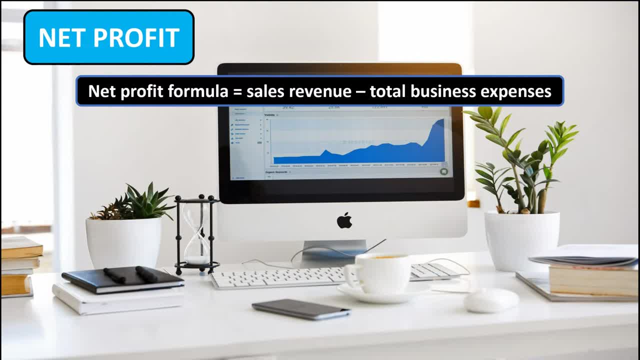 line. It is the amount of money that the business is left with after they subtract their total business expenses from their total revenue. as you can see from the formula that's on your screen now, However, a business's net profit doesn't include any tax payments, as the tax a business 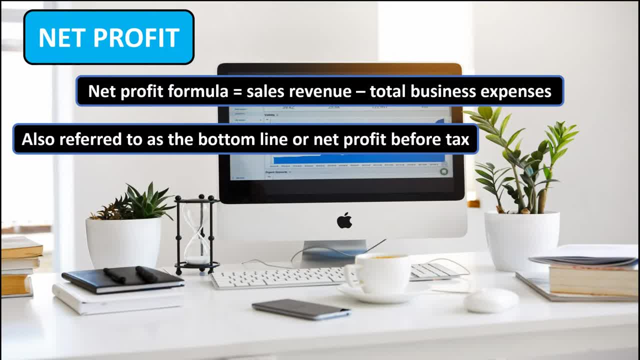 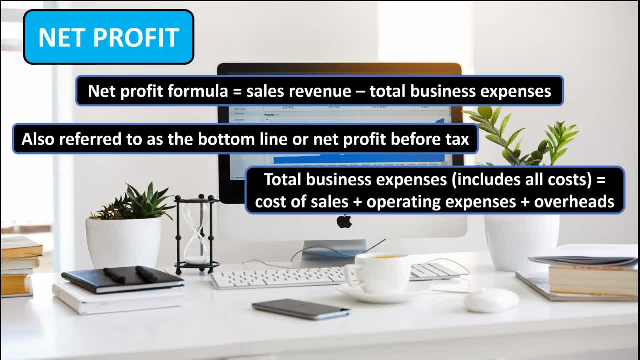 pays is actually based on their net profit figure. Therefore, you may also see this called net profit before tax. The net profit figure appears at the bottom of the statement of financial position. Therefore, the total business expenses include the cost of sales figure used in the gross profit calculation. 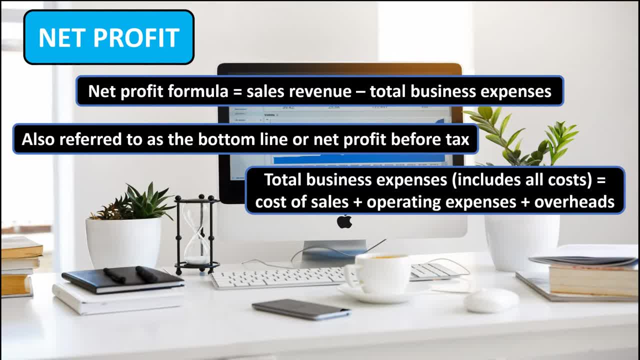 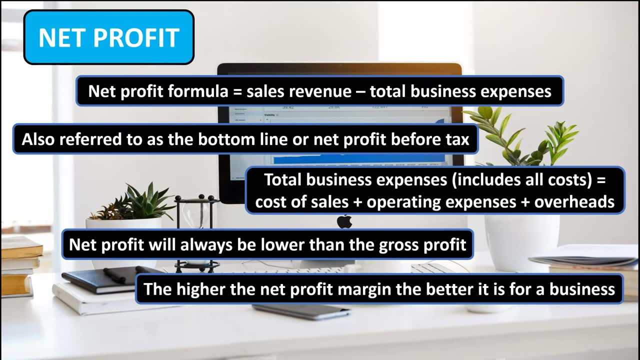 but also includes all other costs, such as the operating expenses and all other overheads that are incurred by the business. The net profit will always be lower than the gross profit. The higher the net profit margin, the better it is for the business, As this shows how profitable the business is overall. 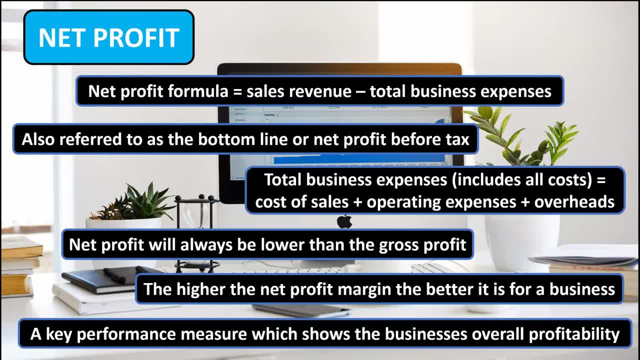 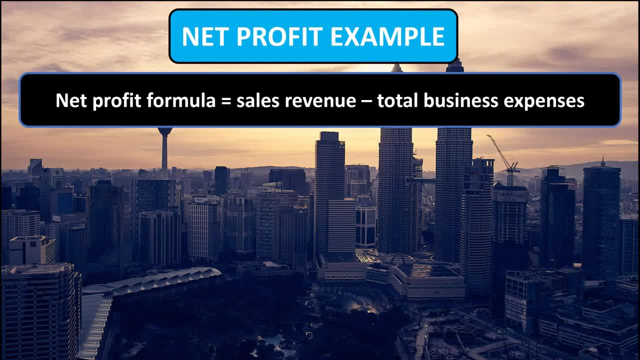 a key measure for any business and something that stakeholders would be interested in. So let's take a look at calculating the net profit, Same as the gross profit. the figures a business requires to calculate their net profit can all be found on their income statement. 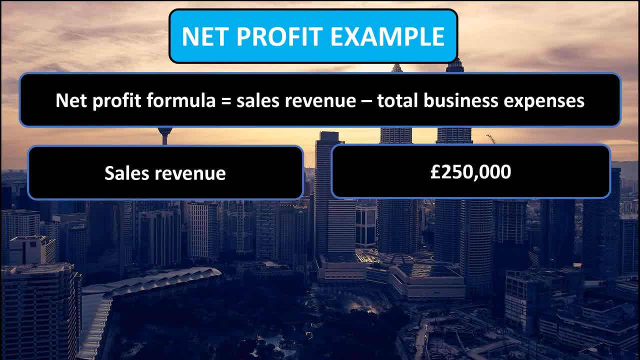 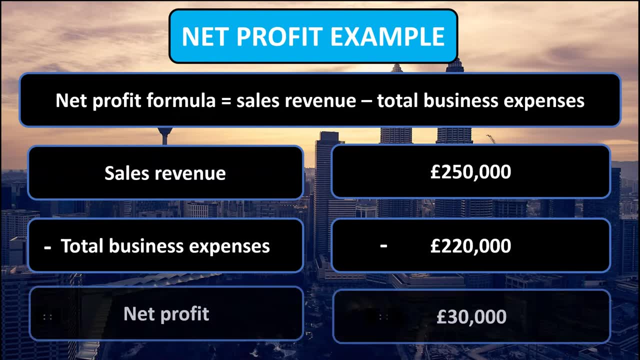 Firstly, we start with the sales revenue, Which in this example, is £250,000.. We then deduct the total business expenses, which in this example, is £220,000.. This leaves us with £30,000.. This is our net profit. 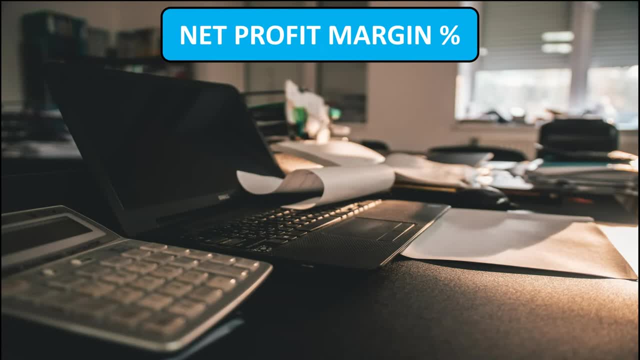 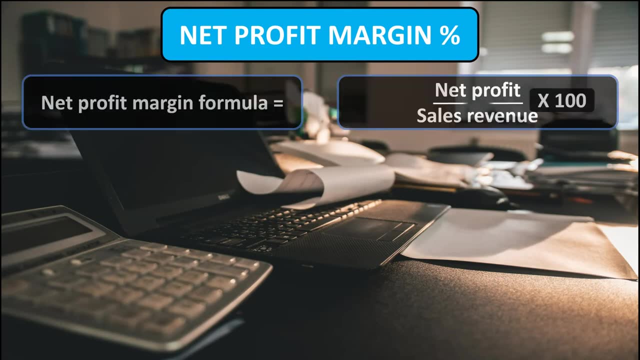 Once a business has calculated its net profit, it can now work out its net profit margin, which is shown as a percentage in the same way that the gross profit margin is shown as a percentage. The net profit margin is calculated by dividing the net profit of the business by their sales. 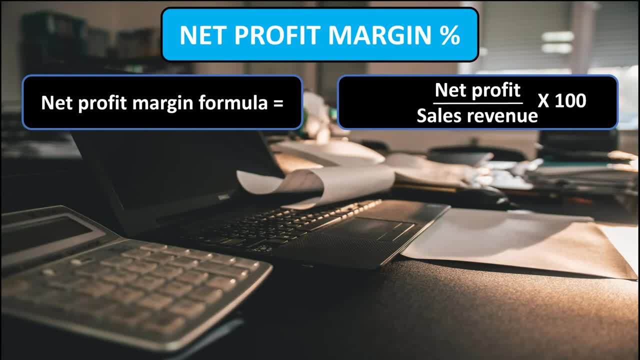 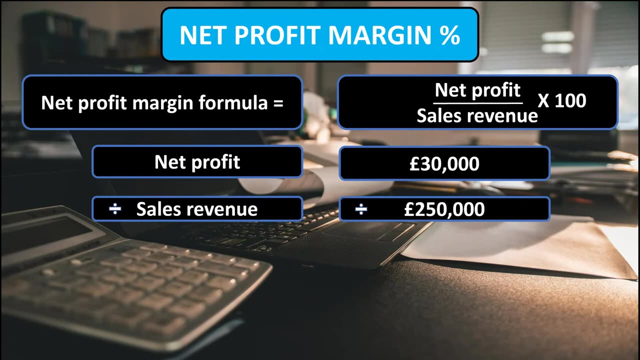 revenue, multiplying the answer by 100, as shown by the formula on your screen right now. So, if we use the figures taken from the previous example, this would require us to start with a net profit of £30,000.. We would then divide this by the sales revenue, which is £250,000. 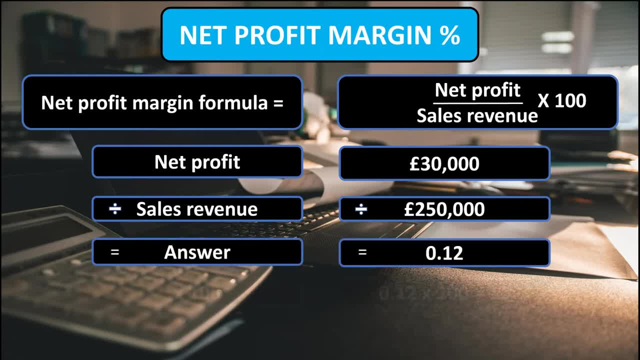 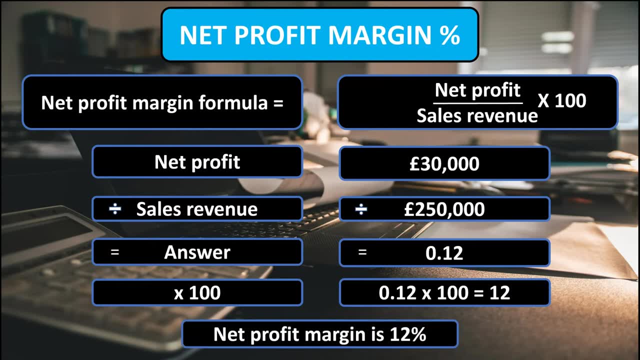 and this would give us an answer of 0.12.. Now it's very important to remember to multiply the answer by 100, which, in this example, gives us 12.. This is your net profit margin. remember it's shown as a percentage, so it's 12%.